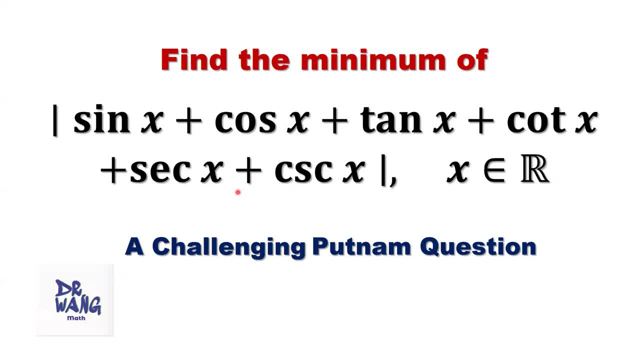 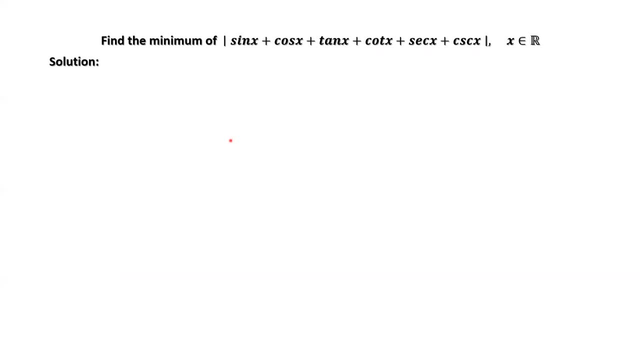 To find the minimum value of this expression. the question is how to convert these six trig functions into one function, cosine. We define f as the inside part of the absolute value. In the first step, we can rewrite the expression. We can write each function in terms of sine and cosine. 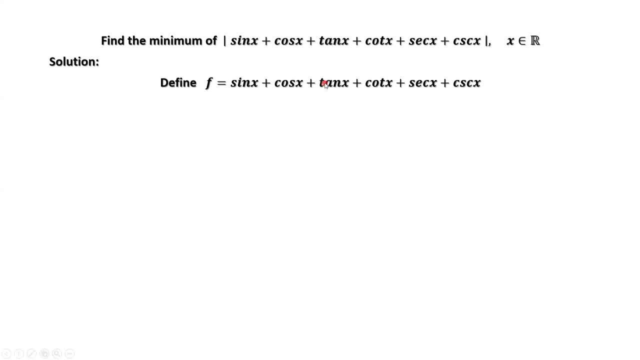 Tangent equals sine over cosine. Cotangent equals cosine over sine. Secant equals one over cosine. Cosecant equals one over sine. The question is to find the minimum value of the absolute value of f. after we define f, We can simplify the sum of middle two terms and the last two terms. 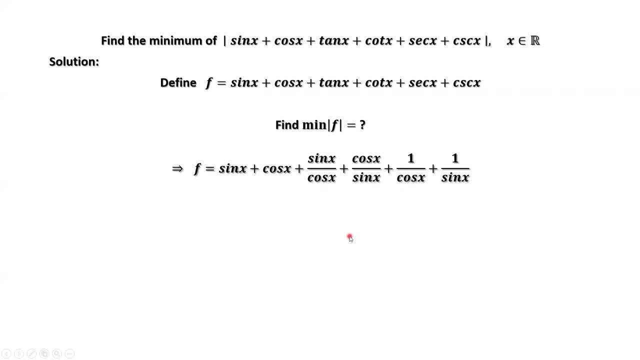 We consider the common denominator, which is cosine x times sine x, The numerator is sine squared plus cosine squared. The numerator here is sine x plus cosine x. From the basic result for sine and cosine we have: sine squared plus cosine squared equals one. 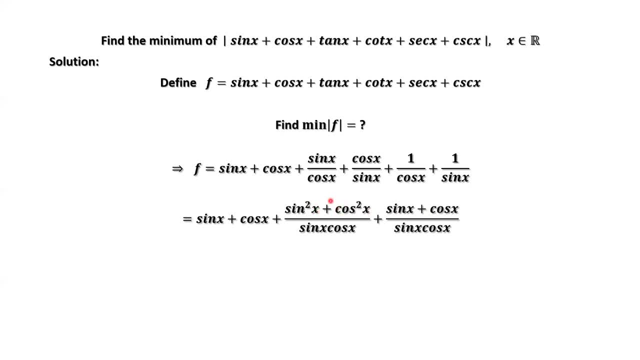 Sometimes we also call this is a Pythagorean result. The denominator of the second equation is one over sine. In this expression of f we have two terms, That's sine x plus cosine x times cosine x. The question is: to what can we convert this sine x plus cosine x and sine x times cosine x? 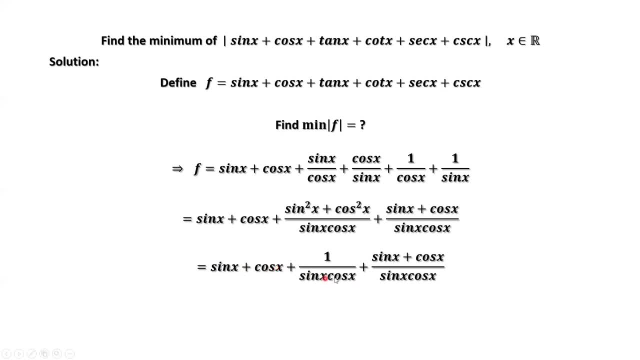 into one constant. The answer is yes, Because this is the problem. We are looking for the constant here In terms of cosine. let's consider sine x plus cosine x. This equation is always true. You can simply check the algebra here. 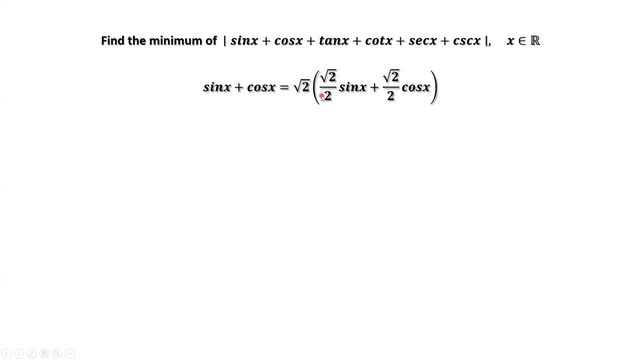 Square root of 2 times square root of 2 over 2,, which is 1.. Square root of 2 times square root of 2 over 2 is 1.. Why are we doing this? We can rewrite square root of 2 over 2 as cosine of pi over 4,. 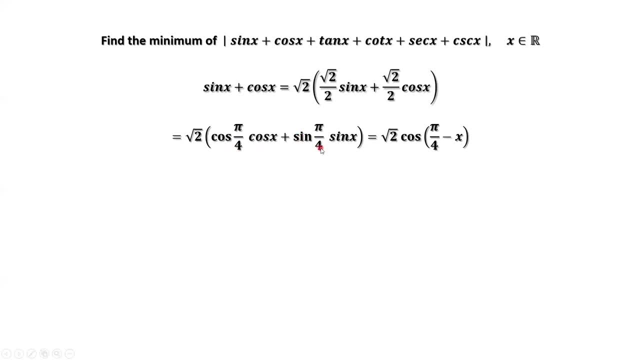 as sine pi over 4.. Based on the difference formula of cosine, we have cosine cosine sine sine. here's plus. The second part is cosine of the first angle minus the second angle. We have square root of 2 outside. 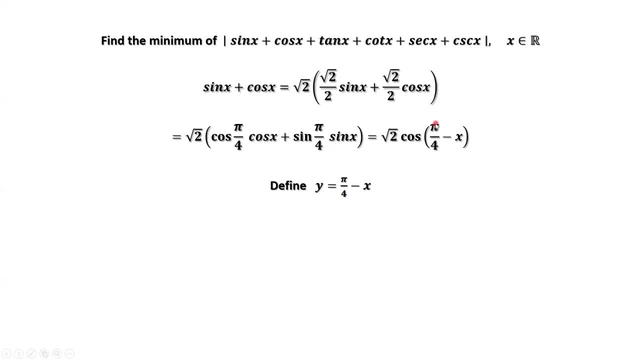 If we define y equals pi over 4 minus x, then we have sine x plus cosine x equals square root of 2 times cosine y. Now we converted sine x plus cosine x into cosine. Let's convert sine x times cosine x. This is simple algebra. 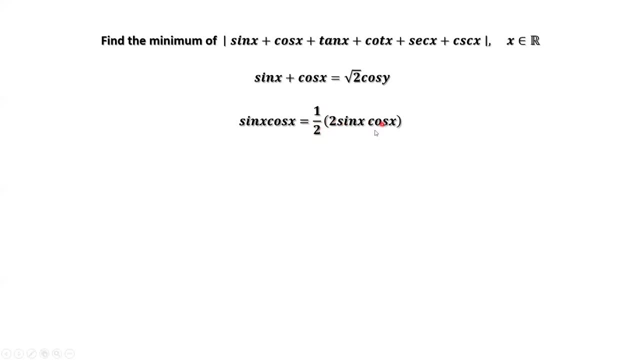 1 half times 2 is 1.. What is the inside part of this parenthesis? This is the double angle formula, which is sine 2x. The question is: can we convert sine into cosine? Yes, Sine equals cosine half pi minus this angle. 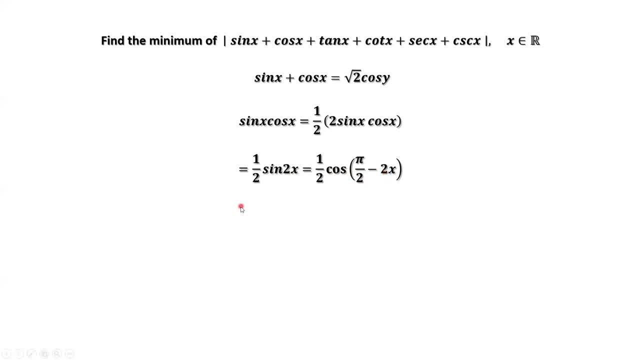 We can factor these two out. This is pi over 4 minus x by definition, which is y. Therefore, sine x times cosine x equals 1 half times cosine 2y. Now we are ready to rewrite f in terms of cosines. 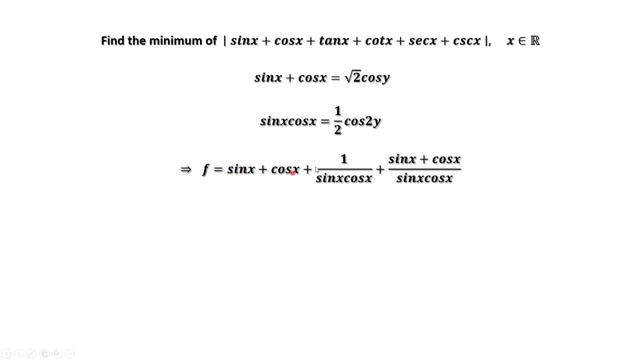 Sine plus cosine equals square root of 2 times cosine y. Here we can replace it by square root of 2 times cosine y. The denominator we can replace by this one. We have the same denominator. We can put 2 in the numerator. 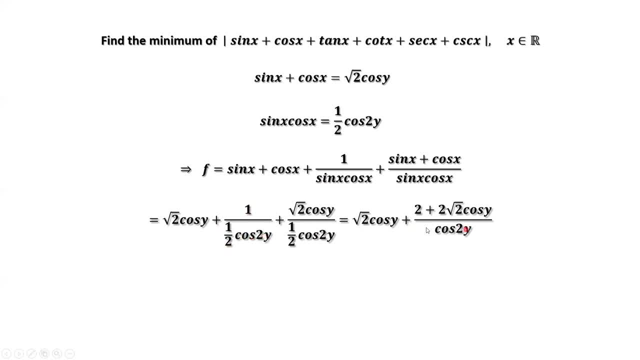 The denominator is cosine 2y, Cosine 2y. Merge the last two terms together, We can factor 2 out. We can define c as square root of 2 over cosine y, Square root of 2 times cosine y. 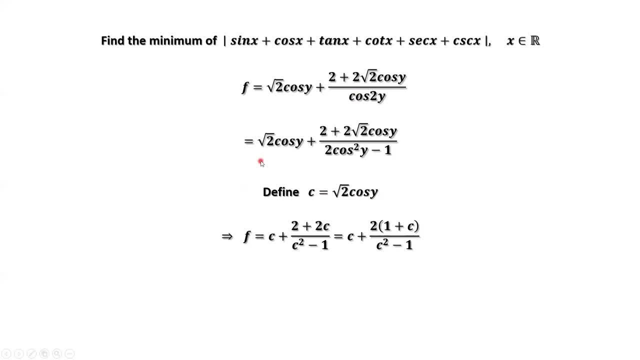 Square root of 2 times cosine y. From here to here we use the double angle formula: Cosine 2y equals 2 cosine y, squared Square root of 2, we can consider that 2.. We can consider that as square root of 2 squared. 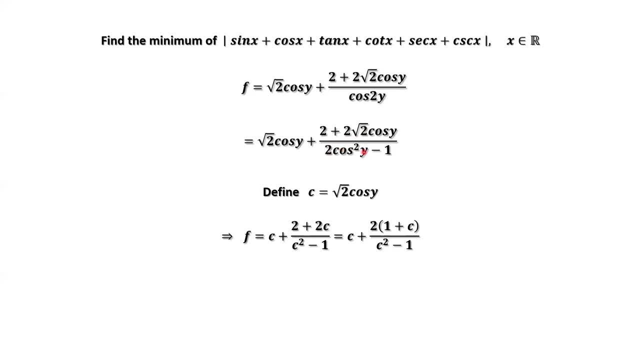 which is square root of 2, cosine y, then squared, That means we have c squared here. Now we factor 2 out The denominator, that's c minus 1 times c plus 1.. c plus 1 here can be canceled. 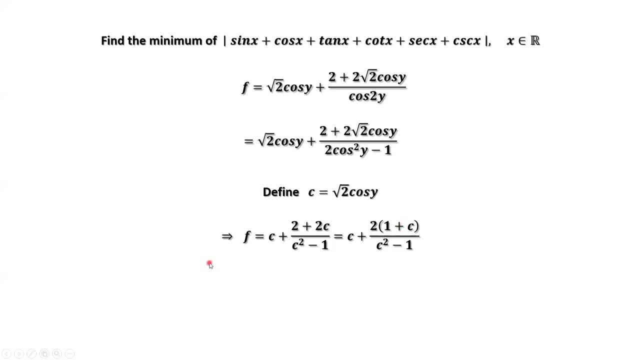 from both numerator and denominator. Then we have f equals c plus 2 over c minus 1.. So here c cannot be 1.. If c equals 1, f equals infinity. We only care about the minimum value, not maximum. So here: 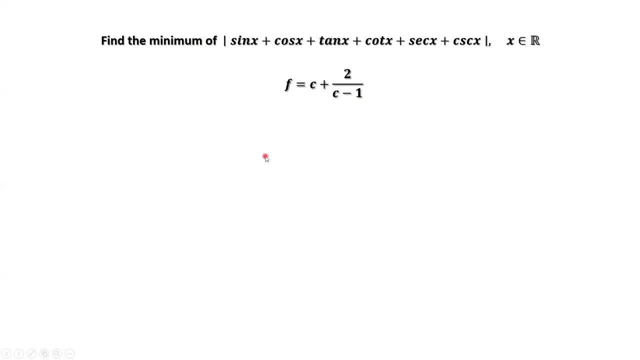 we don't consider c equals 1.. Only two other situations we need to consider. The first situation: is c bigger than 1.. Then we will discuss c less than 1.. If c is bigger than 1, the absolute value of f equals. 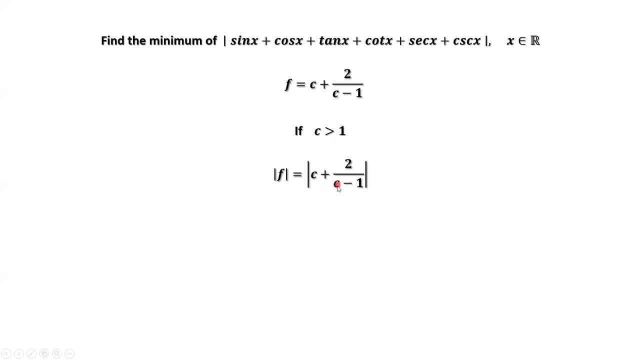 the absolute value of c plus 2 over c minus 1.. Because c is bigger than 1, the denominator is positive. The inside part is positive. Therefore we can directly drop the absolute value sign. The absolute value of f equals c plus 2 over c minus 1.. 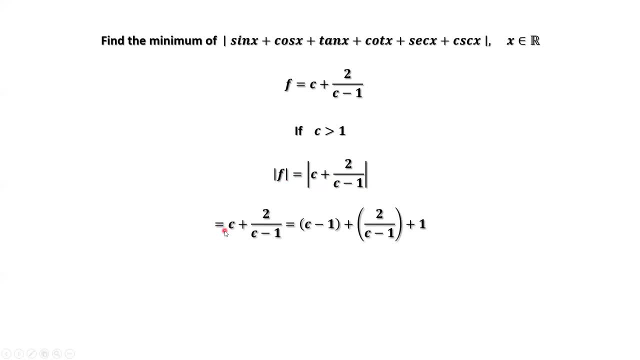 The absolute value of f equals c plus 2 over c minus 1.. We put the negative 1 here plus 1 here to keep the balance. Why are we doing this? We are going to use an important formula to derive the lower bound. 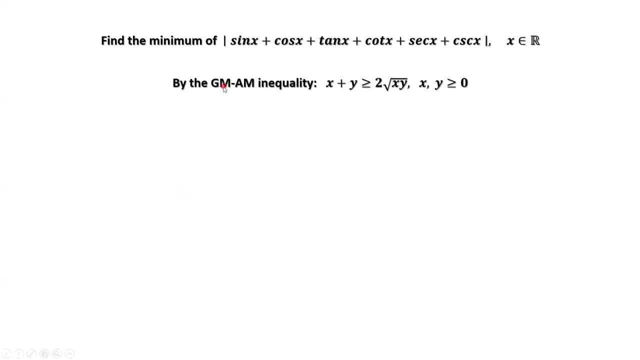 By geometric means and arithmetical mean, inequality. This is the inequality If x and y are bigger than or equal to 0, x plus y is bigger than or equal to 2 times square root of x times y. Originally, 2 is here. 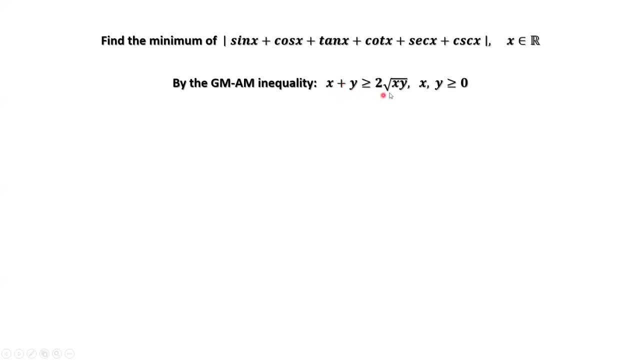 x plus y over 2, that's the arithmetical mean. Square root of x times y, x times y is the geometric mean, The sum of the first two terms. we can use this inequality: x, in our case, is c minus 1.. 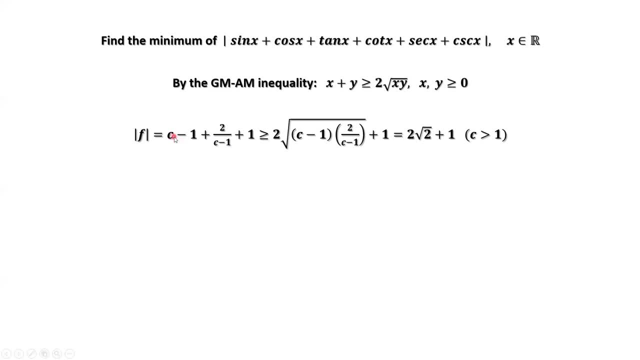 y is 2 over c minus 1.. c minus 1 here is positive because c is bigger than 1.. Apply this formula: the inside part, c minus 1 and c minus 1, from the denominator can be cancelled out. We only have 2 left inside of the square root. 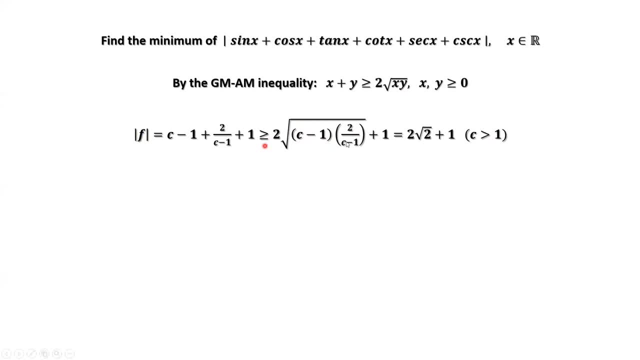 Therefore, the absolute value of f is bigger than or equal to 2 times square root of 2 plus 1.. This is the lower bound. When c is bigger than 1, we also need to consider c is less than 1.. 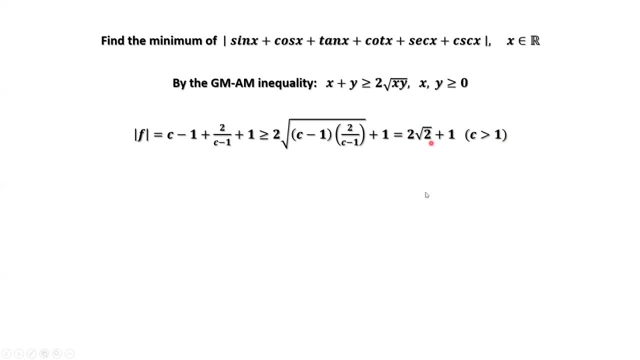 Find the lower bound, Then compare which one is smaller. If c is less than 1, we rewrite the inside part as 1 plus c minus 1 plus 2 over c minus 1.. So here minus 1 plus 1, cancel. 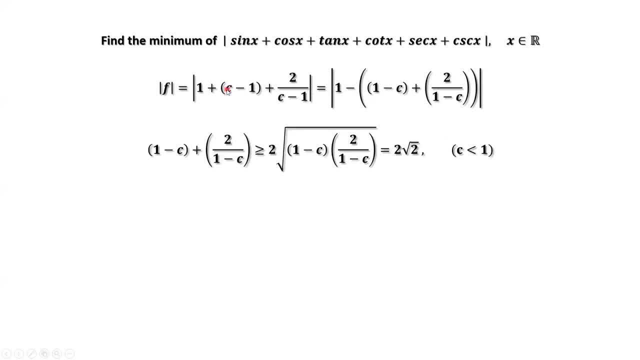 Then we swap the locations of c and 1.. So 1 minus c, 1 minus here, c minus 1. If we swap, we have to put the negative sign in front. Now the inside part is different. There is a difference of 2 parts. 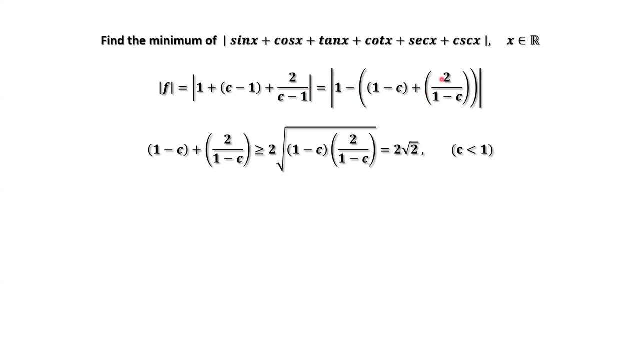 What are we doing here? We want to check if the inside part is positive or negative. Check the second part. This is the second part, because c is less than 1.. 1 minus c is bigger than 1.. 1 minus c is bigger than 0.. 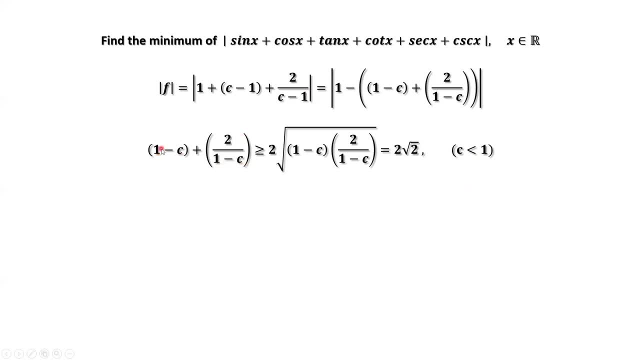 1 minus c is bigger than 0. Therefore the condition of the inequality is satisfied. Then we have the result. Apply the inequality for the sum of the first two terms, which is big Zn, or equal to 2 times square root of 2.. 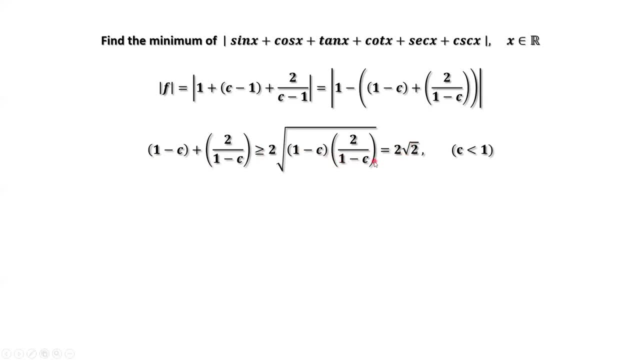 Similarly, here we can cancel 1 minus c, 1 minus c from both numerator and denominator. Now look at the inside part, 1 and the second part. The second part is bigger than 2 times square root of 2,. 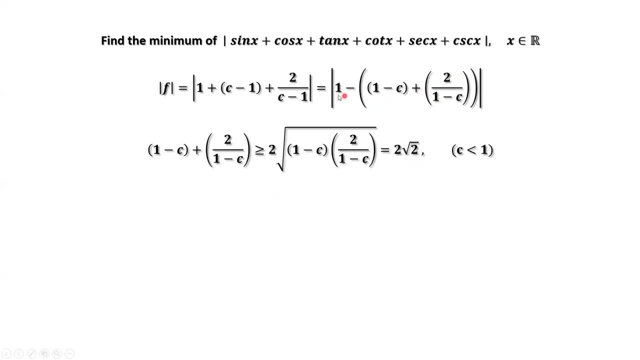 which is bigger than 1.. So the second part is bigger than 1.. The difference is negative. How to drop the absolute value sign? if the inside part is negative, We have to put the negative sign in front. Negative 1,. 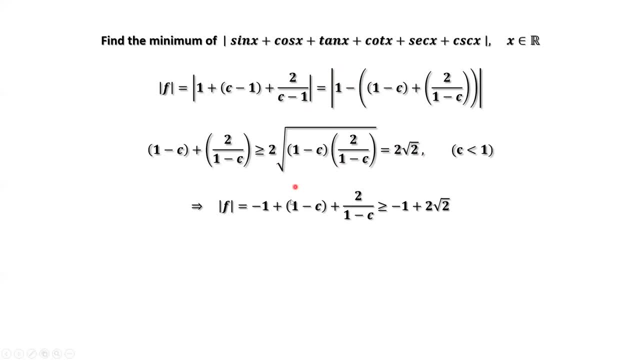 negative: 1. Negative, negative become positive and become positive. Now look at the sum of the last two terms. We use this result again. What is this result? This part is big Zn, or equal to square root of 2 times 2.. 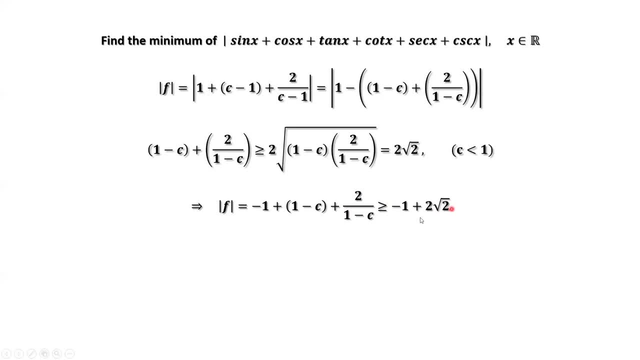 This lower bound is smaller than the one we derived before, So we should use this one. This is just a small bound. The question is: is it reachable? Next thing we need to do is to check if we can find the Z such that. 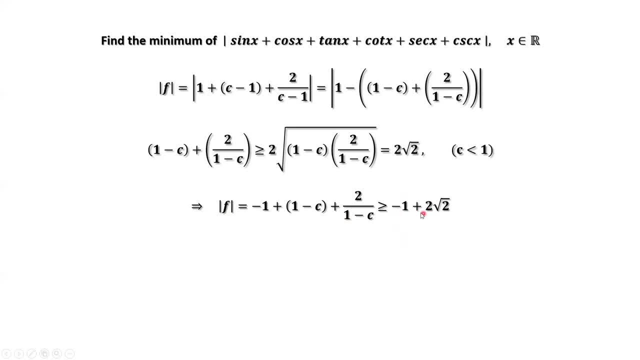 the absolute value of F equals negative 1 plus 2 times square root of 2.. By our definition, Z equals square root of cosine y, y as defined as pi over 4 minus x. Therefore, the Z value is between square root of 2 and. 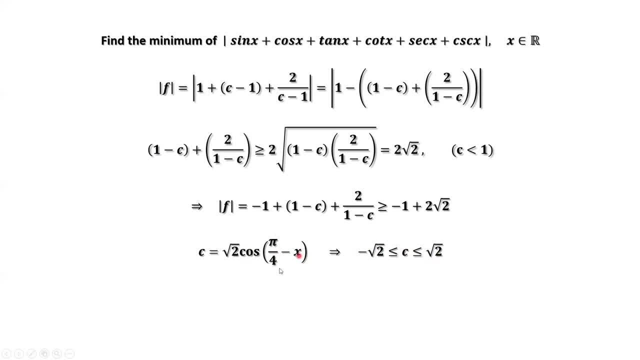 negative square root of 2. Because the maximum value for cosine is positive. 1. The minimum value for cosine is negative. 1. We only need to find the Z value inside of this interval, such that the absolute value of F is equal to. 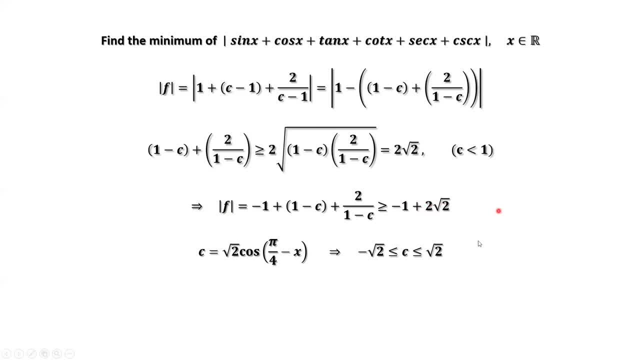 negative: 1 plus 2 times square root of 2.. The equal sign is true if x equals y. for this inequality, In our situation, x equals 1 minus c. y equals 2 over 1 minus c. This is a quadratical equation. 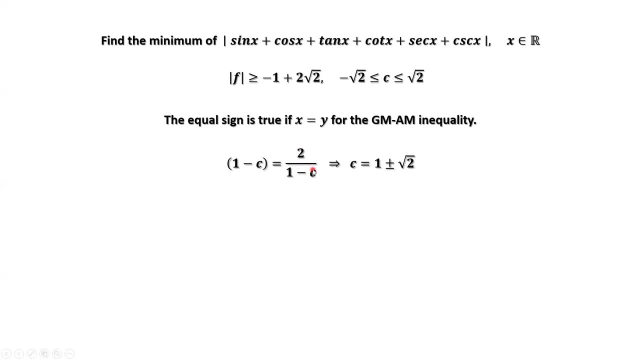 You can simply simplify this equation by both sides, timing 1 minus c, Solving this quadratical equation. we have two values for c: 1 plus square root of 2 and 1 minus square root of 2.. Because we consider: 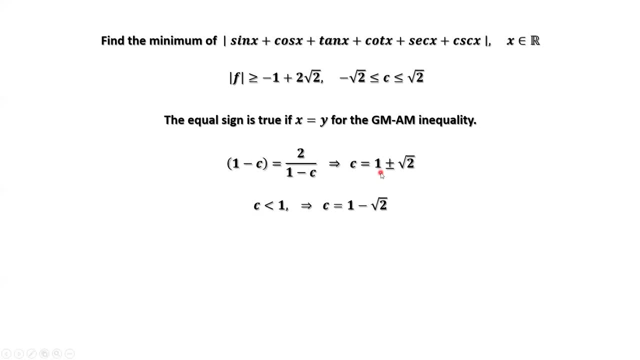 c less than 1 now. So we only have one solution to satisfy our condition. c equals 1 minus square root of 2.. If we replace c by 1 minus square root of 2 in this expression of the absolute value of F, 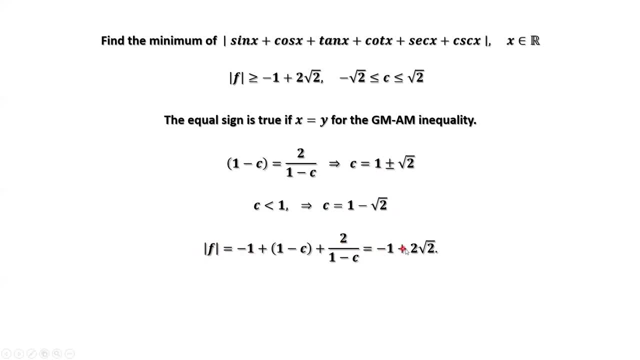 we have the result: negative 1 plus 2 over square root of 2.. This means the minimum value is reachable when c equals 1 minus square root of 2.. The final answer is: the minimum value of absolute value of F equals negative 1 plus 2 times. 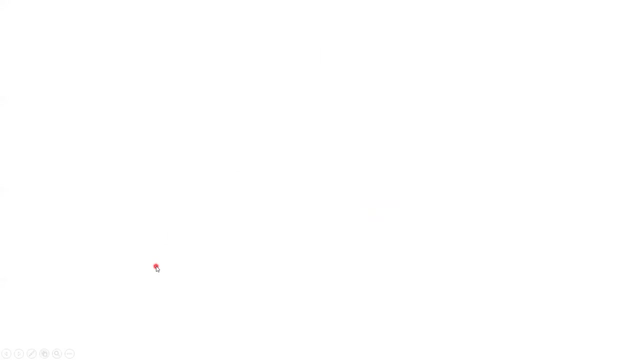 square root of 2.. That's all. Thanks for watching and see you next time. Thank you. 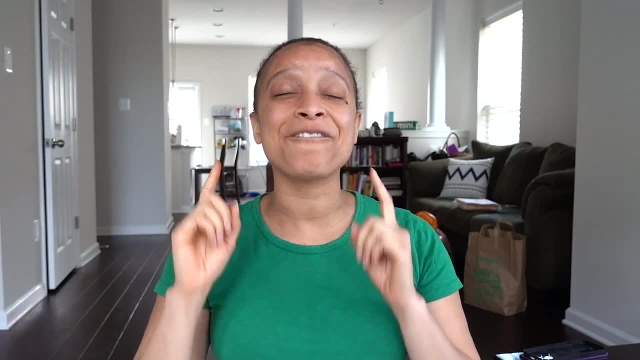 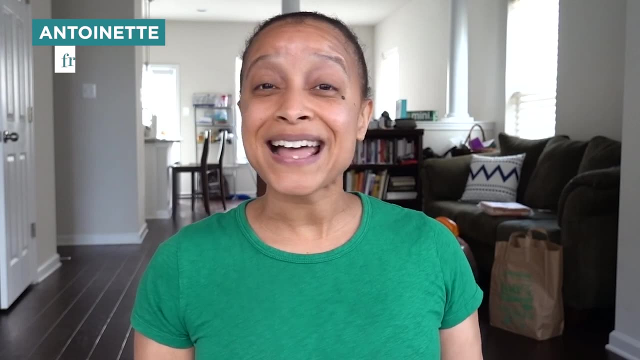 Sailing into the dazzling blue waters of the Mediterranean Sea on my first ever Mediterranean cruise was such a memorable bucket list experience. My name is Antoinette and on my channel I help you plan well, have fun and travel the world. In today's video, I'm sharing with you. 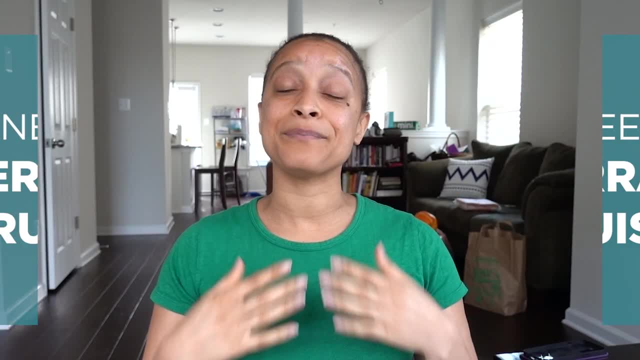 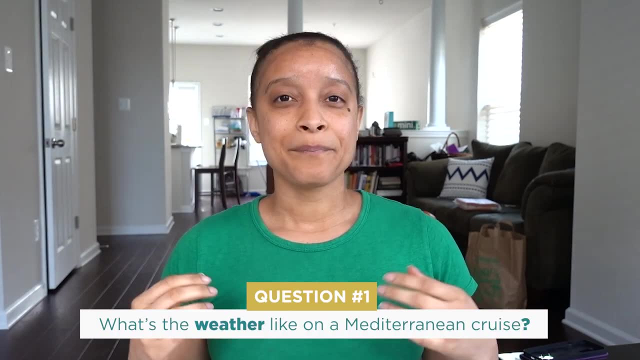 what you need to know before a Mediterranean cruise. based on my experience as a first timer, I had a lot of questions about the weather, so let me answer a few of them right up front. Mediterranean cruises are typically from late April all the way through October, the warmest. 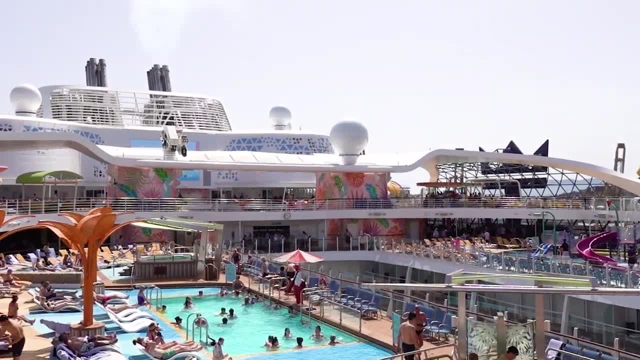 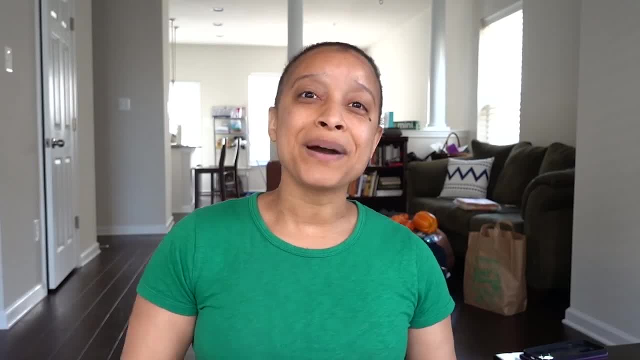 months of the year in Europe, The temperature can reach 80,, 90,, even 100 degrees Fahrenheit, so expect it to be hot. okay, We'll talk about what to wear later in the video, but another question that I had was: is it cold at night on a Mediterranean cruise? And the answer to that is: 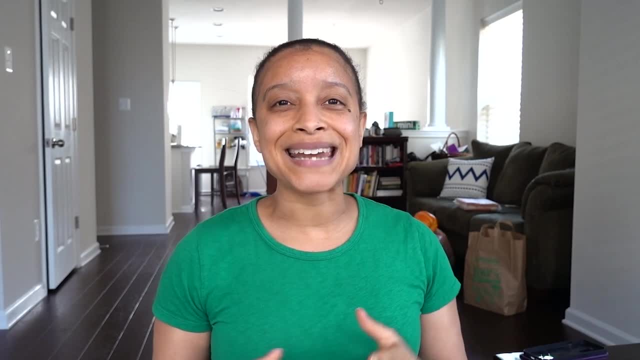 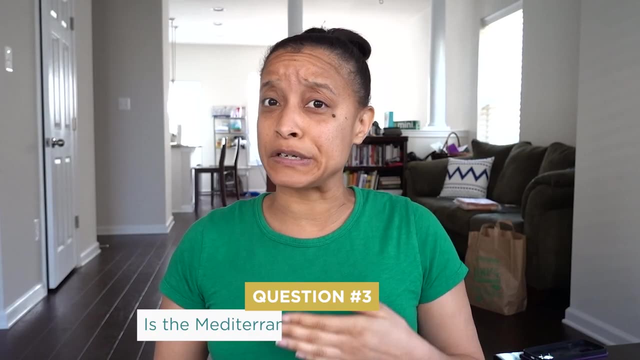 yes, it is cold. As hot as it may be during the day, at night it can be much cooler, reaching 50 or 40 degrees Fahrenheit, so bring a light jacket for evening activities. Is the Mediterranean sea rough for cruising? Are Mediterranean cruises pretty calm, And what?